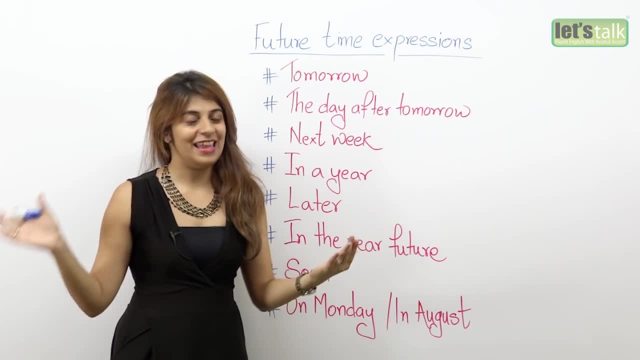 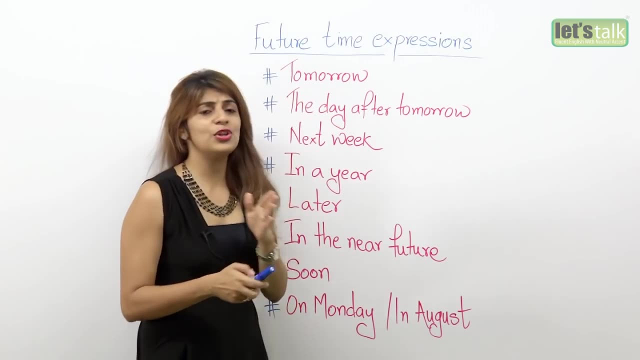 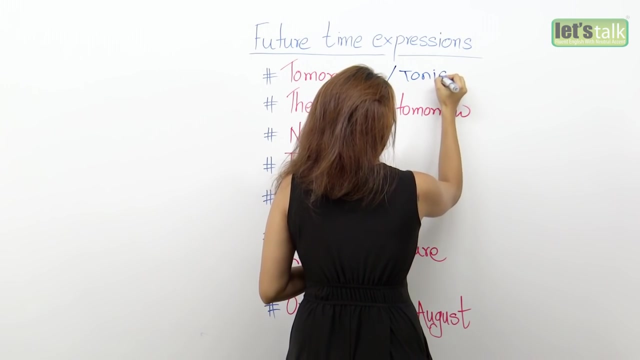 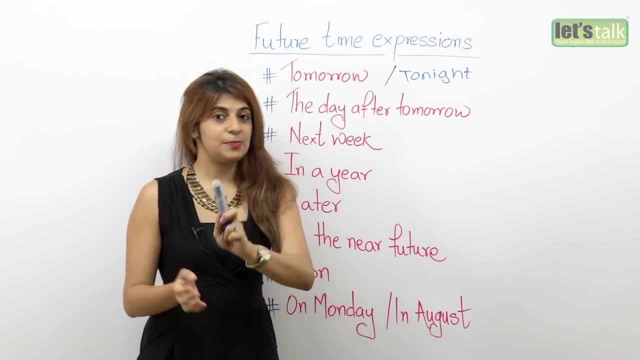 tomorrow. So it's either in the beginning or at the end of a sentence. Got that? So tomorrow is the day after today. You can also use another expression: that is tonight. So tonight I'm gonna go out with my friends. So tonight is another expression that you. 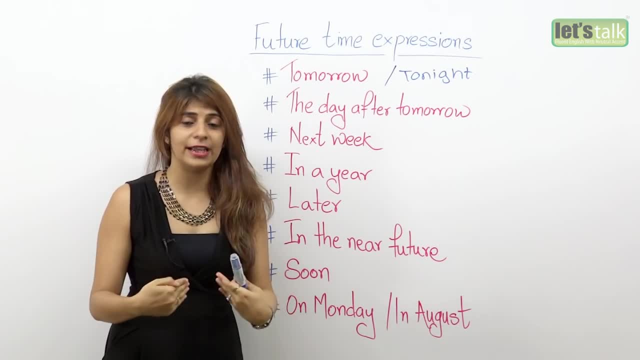 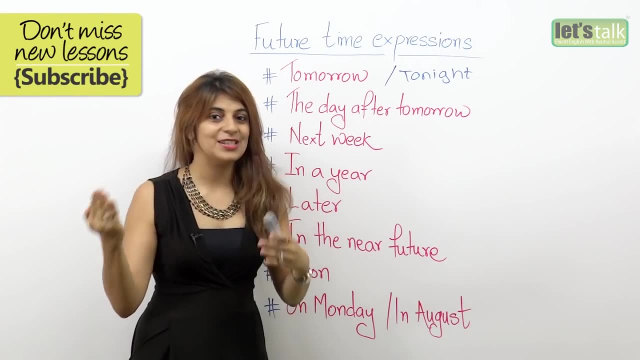 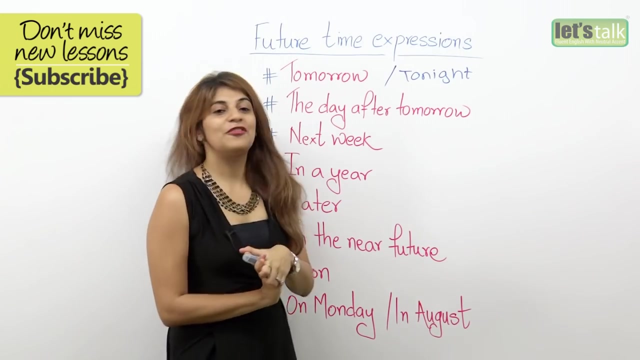 can use for the same day. Now as I'm saying tonight. of course, I'm talking about today, but I'm talking about later time. It's tonight, So tonight is considered to be a time expression of the future. The next one that I have for you is the day after tomorrow. Now the day. 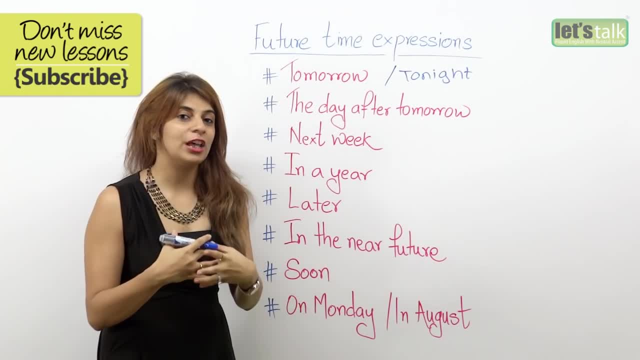 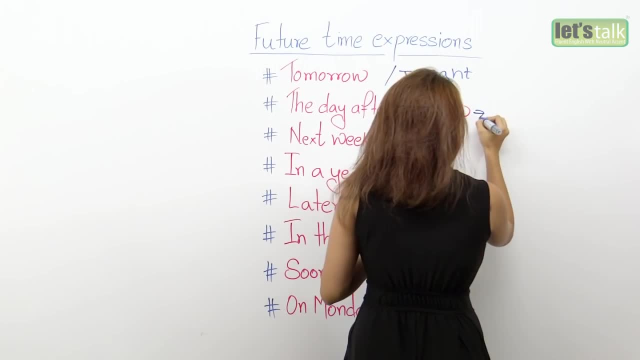 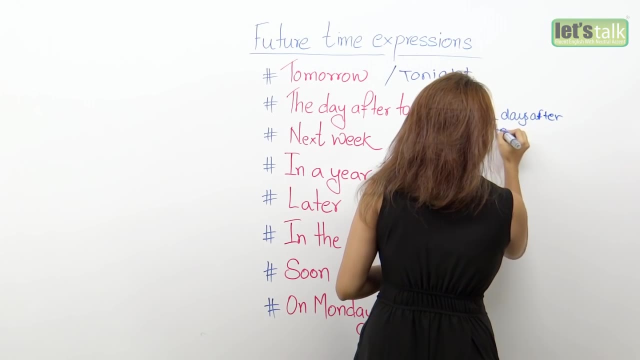 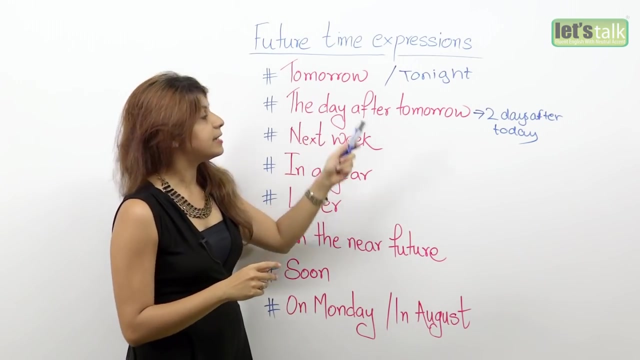 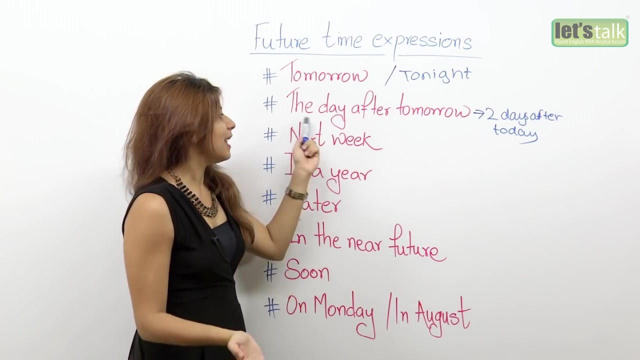 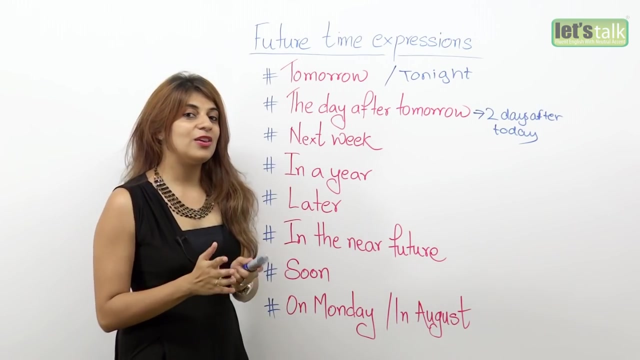 after tomorrow is used when we are talking about a day that is two days after today. My mom is gonna come visit me the day after tomorrow, Or I am going to my uncle's house the day after tomorrow, So that's how you can use this time expression. The next one is next week. Now, when do we use? 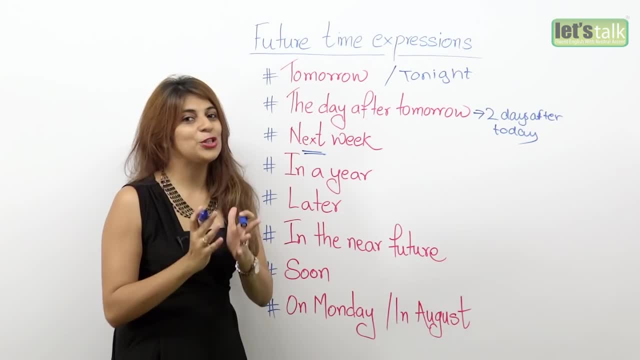 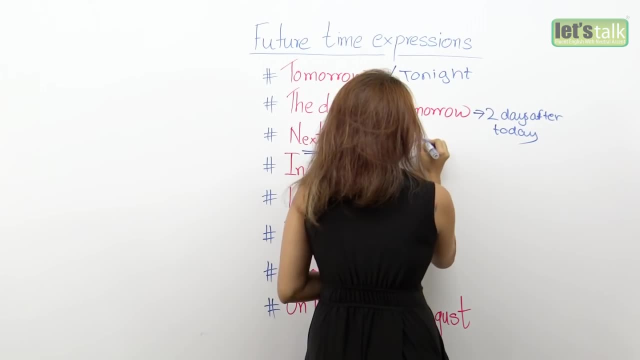 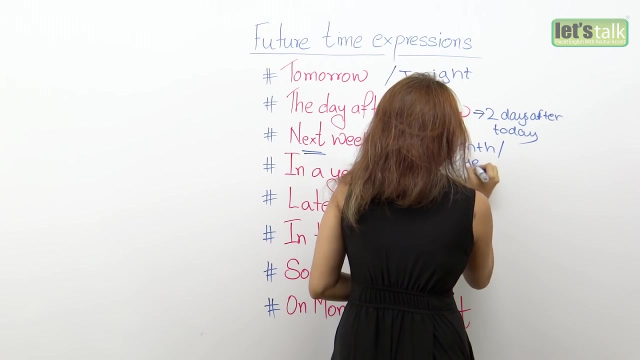 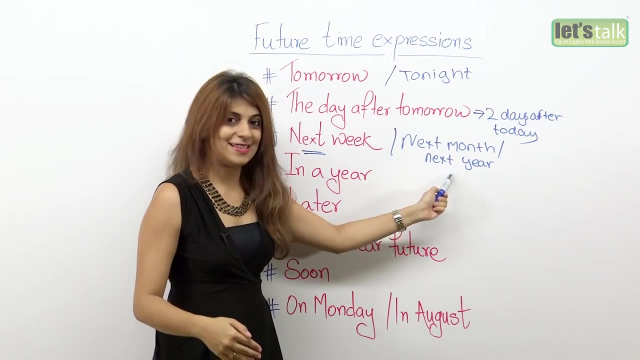 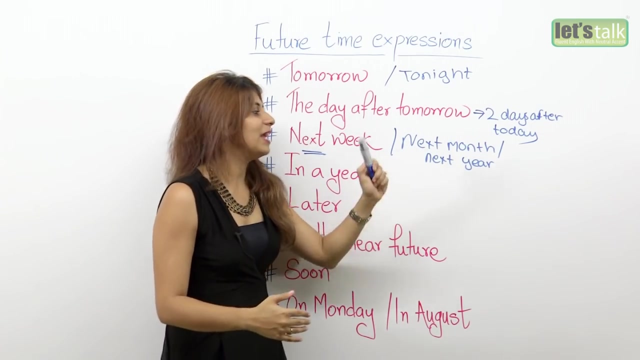 the word next, Of course, when we are talking about future, Now, next week- similar expressions to this one is next month or even next year. So we are not talking about this year, but the year after this one would be next year. I am not talking about this month, but the month after this one would be called as next. 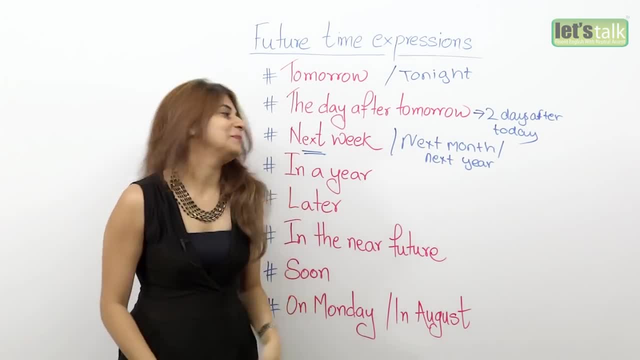 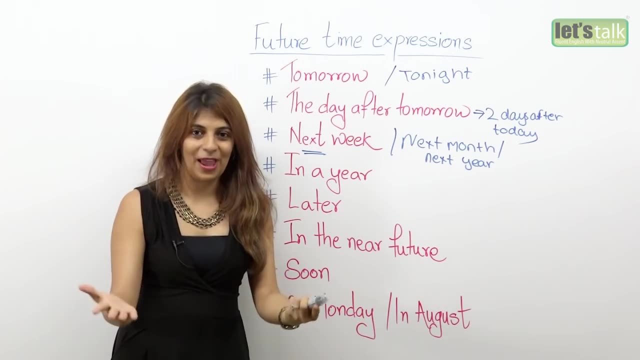 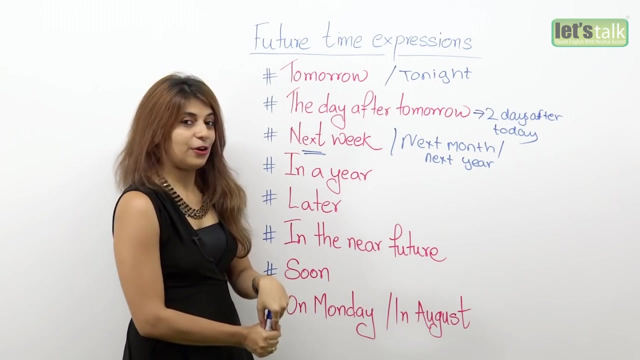 month. Next month, I am flying to Spain. Next week, my friend is coming over to celebrate her birthday, So that's how you can use this expression. Another one that I have for you is in a year. Now, when do you use this expression? Of course, it is a future time expression. 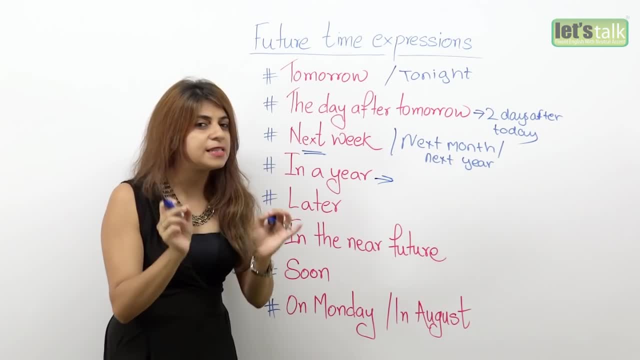 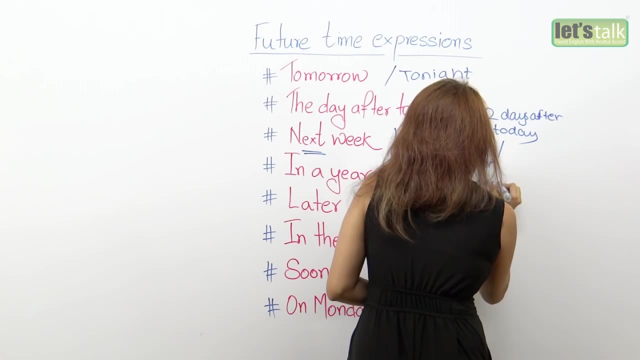 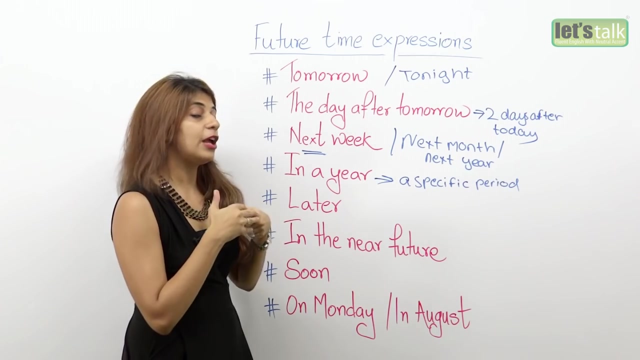 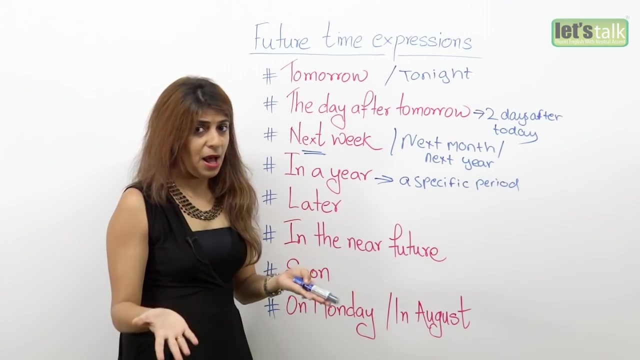 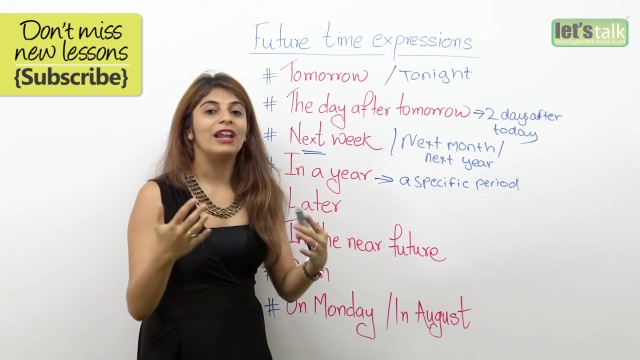 However, it is used when you are talking about a specific period, A specific period in the future. So, for example, she will be a graduate in a year, Or I might finish this course in a year, So it can be in a year. Another expression, a similar expression, is in a month or in a. 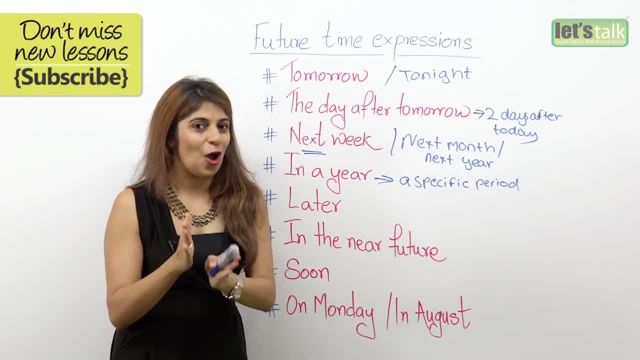 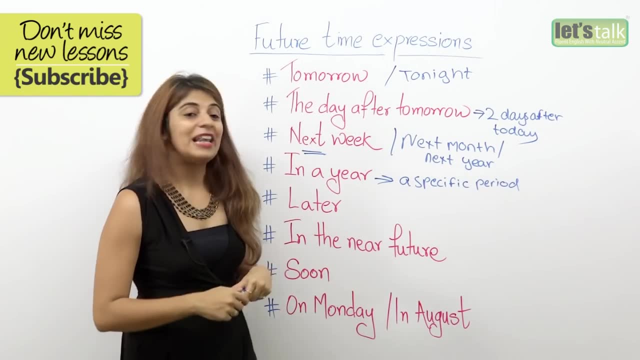 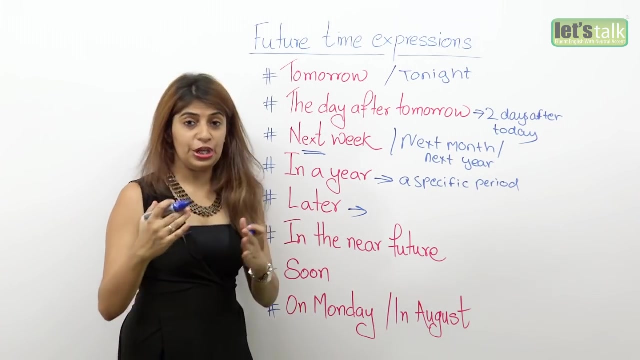 week. So use it when you have to talk about the future, Especially when you are talking about a specific period in the future. The next one later Now, when do you use this expression? Now, later can be either used for the near future or it can be used for the. 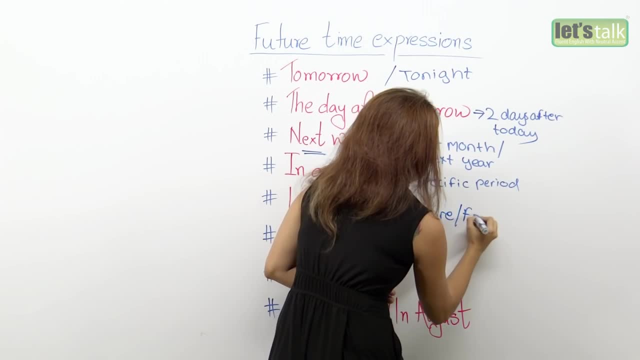 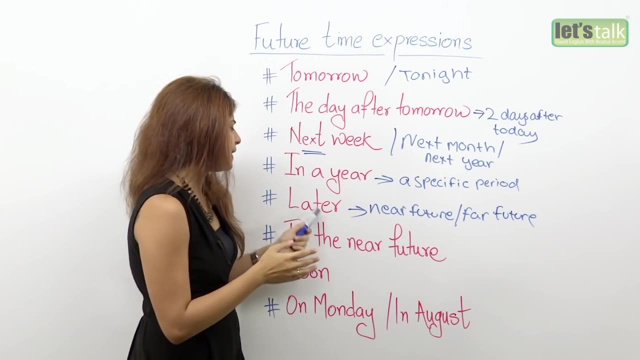 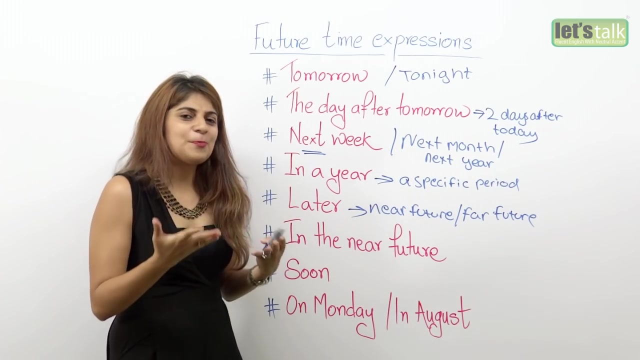 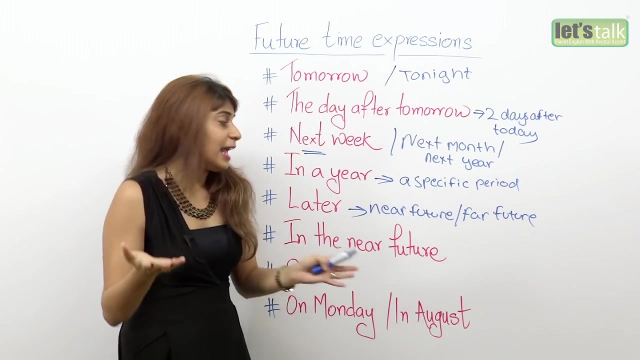 far future. Now, how do you use that? Well, let's talk about an example. I'll see you later. So I'll see you later is probably. I am just talking about a time, not a specific time, but some time in the future. So it can be near future or far future. So either I'll 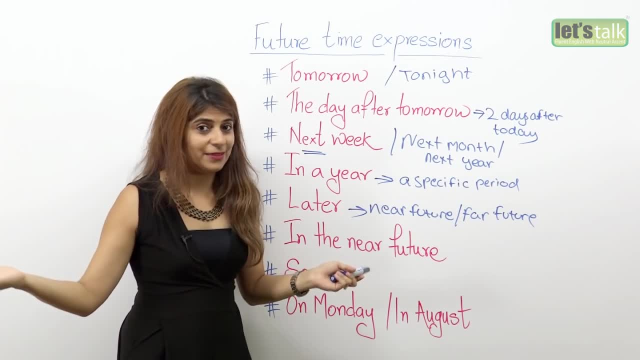 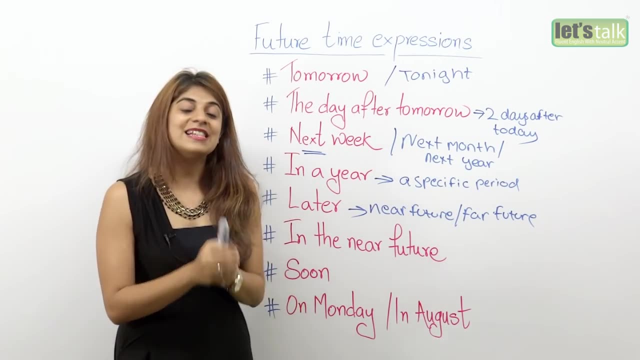 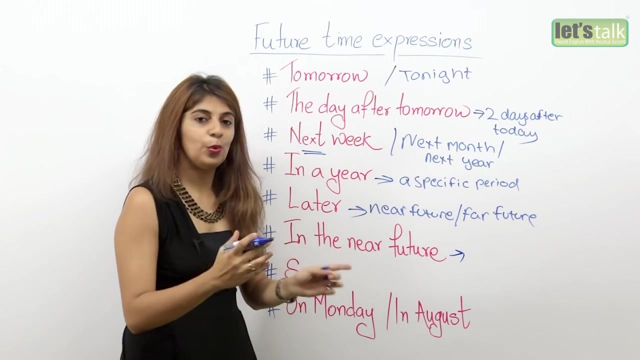 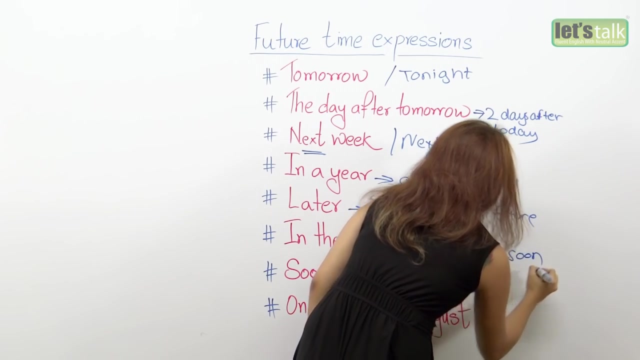 you maybe in two days, or maybe I'll see you in a month, So that's how you use this expression. The next one in the near future. Well, this is a very common expression that's used by many of us, and it actually means that you will see that person very soon, Or you will. 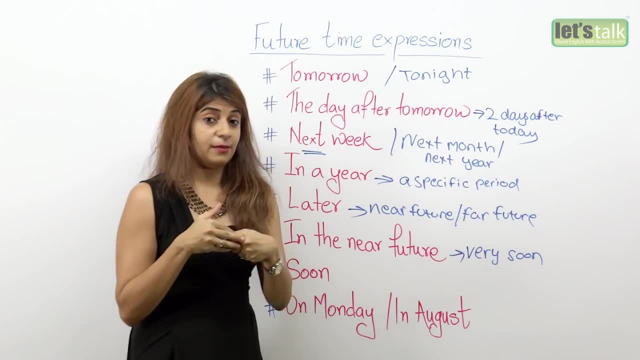 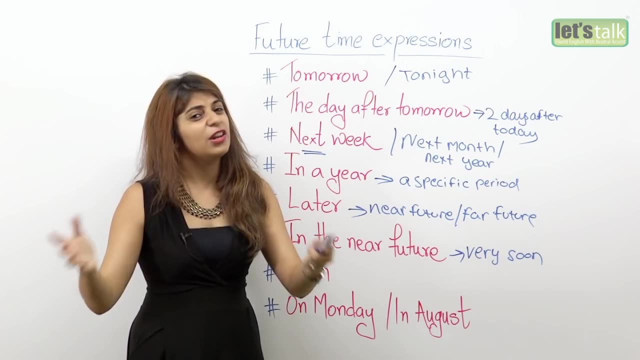 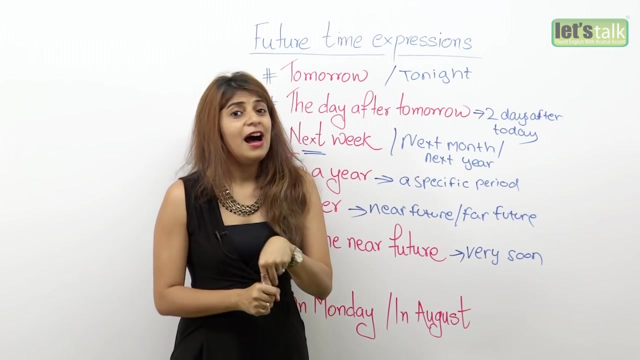 do something very soon. Let's think of an example. Maybe my washing machine isn't working. It's not working that great, my clothes are not being cleaned, So I would say that in the near future I will have to buy a new washing machine. So it means that, because it's not, 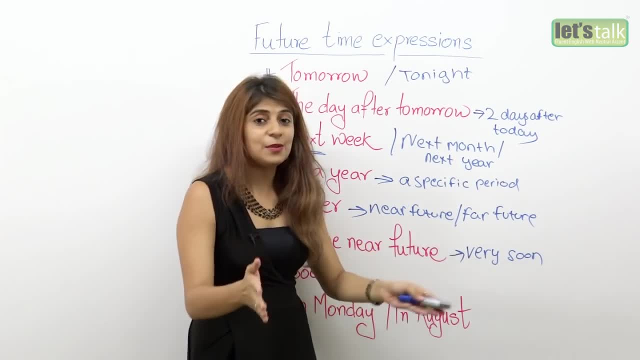 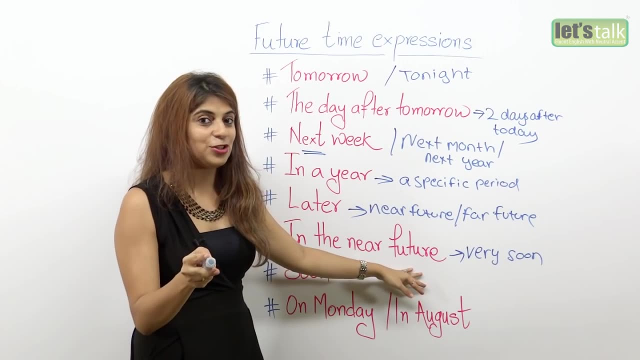 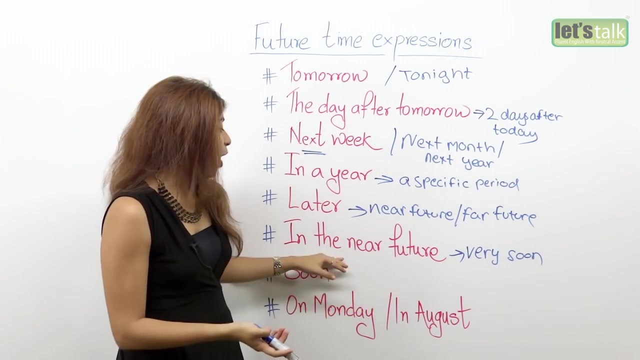 working now. so in the future or very soon, I'll have to buy a new washing machine, So in the near future. you use this expression when you are talking about doing something or meeting someone very soon. I hope to see you. in the near future It means I hope to.